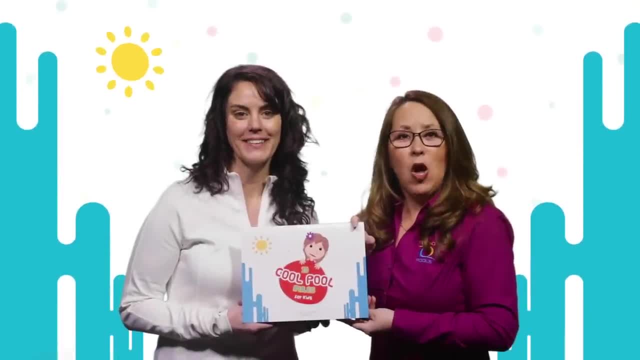 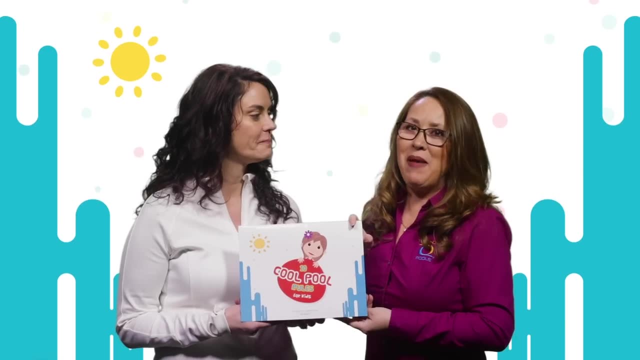 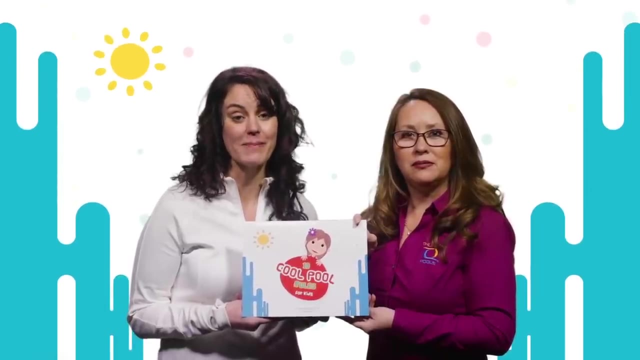 Hi kids. I'm Pilar And I'm Annie. We're from Thursday Pools and our company makes fiberglass swimming pools. Did you know that May is the water safety month? It is Pilar, So that means it's time to think about how to have fun and be safe in the water, because swim season is coming. 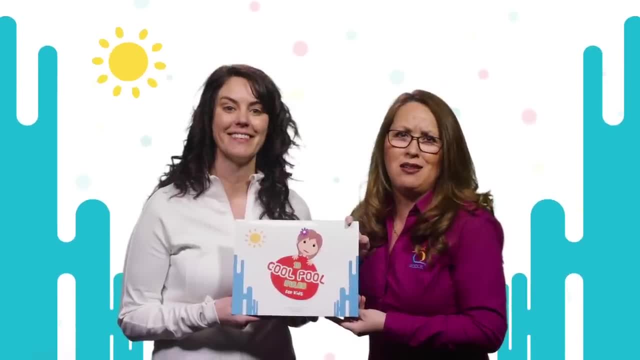 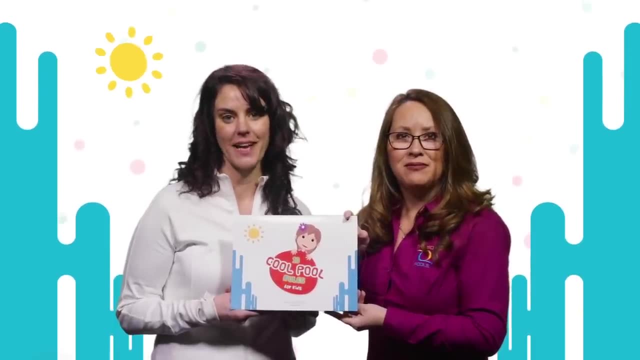 How many of you like to go swimming when it's hot outside? Yes, a lot of you do. We do too. So how about if we have some fun today while we read this book together? It's called Ten Cool Pool Rules for Kids. 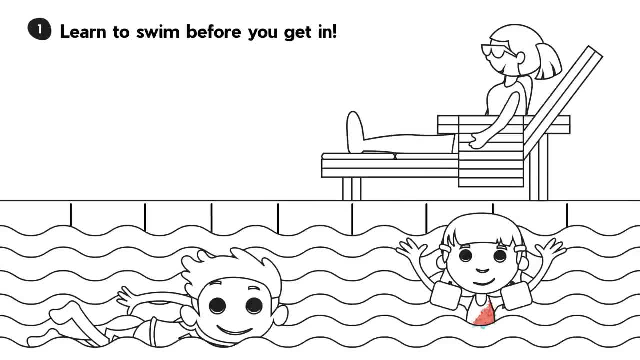 Rule number one is learn to swim before you get in. You might see other kids swimming and think it looks easy, but you need to stay in the shallow end and wear swim floats until you're a strong swimmer. Also, never push another kid into the pool. You don't know if they can swim or not. so it's not a good joke to play. 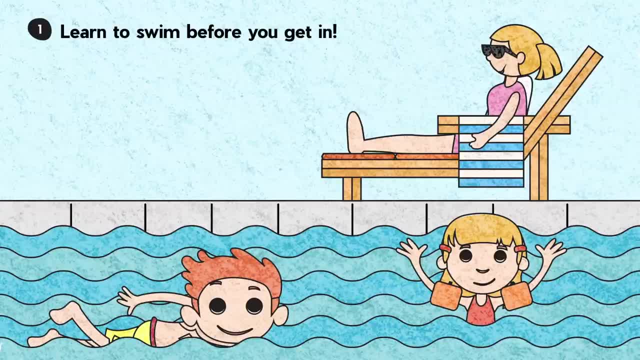 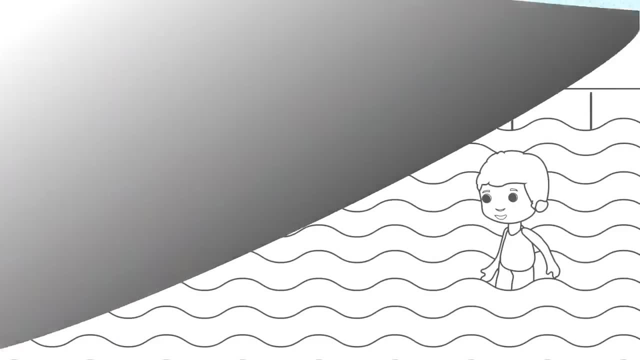 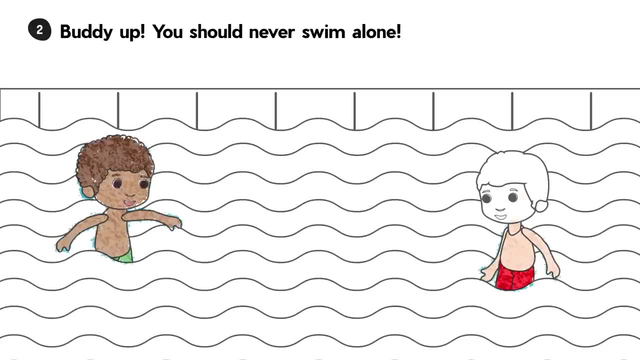 So rule number two? Rule number one is: learn to swim before you get in, That's right. And rule number two is: buddy up. You should never swim alone or go into the water unless there's an adult with you. Plus, you can't play Marco Polo by yourself anyways. 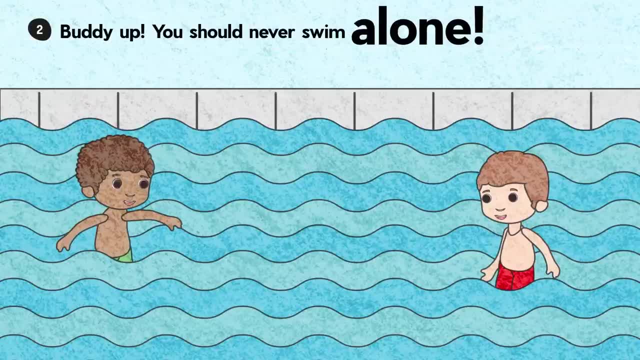 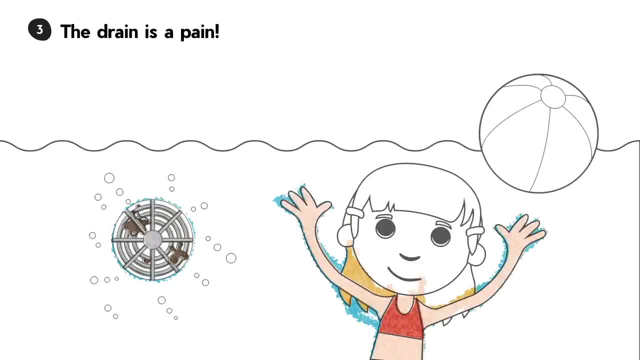 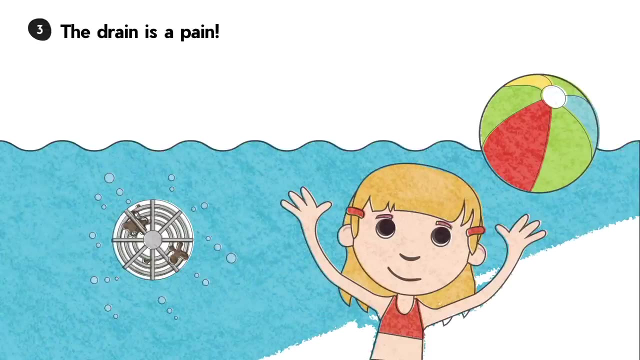 So remember: never swim alone. Great job. Here's rule number three: The drain is a pain. Always stay away from the drain. It's a dangerous place to play because the water going down through it causes a strong pull and it can catch your fingers, toes, swimsuit or hair. 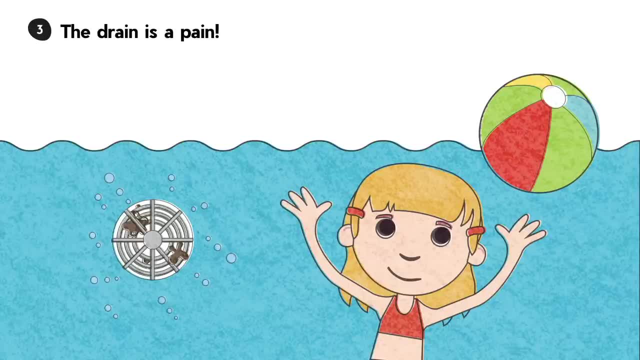 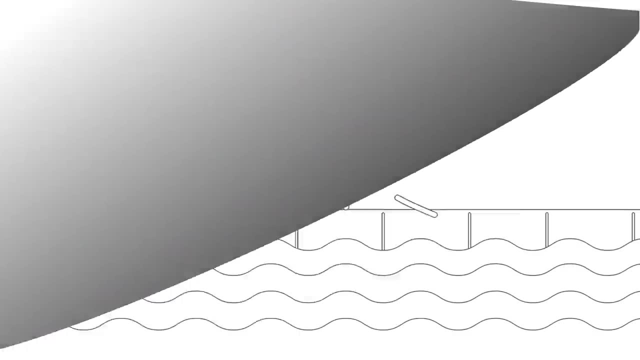 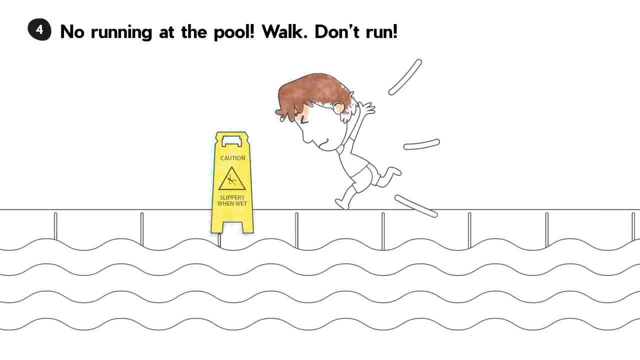 So stay away from the drain and you'll be fine. So what's the drain? A pain, You got it. Rule number four is no running at the pool. Your teachers probably tell you not to do this in the holes too, don't they? 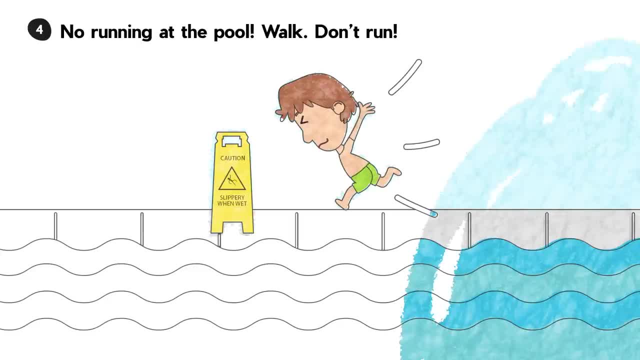 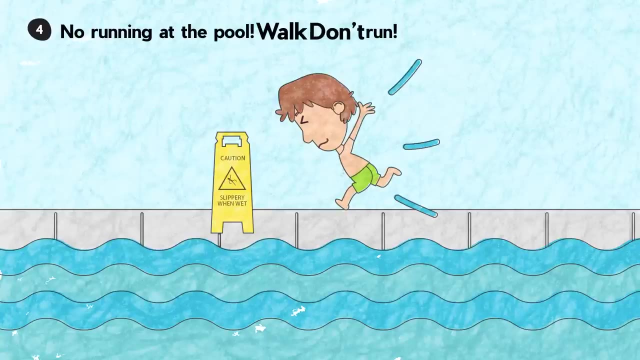 Well, around the pool the deck can be very slippery when it's wet. You certainly don't want to sleep and fall and then have to sit on the sideline while your friends swimming. So when you're at the pool, walk, don't run Exactly. 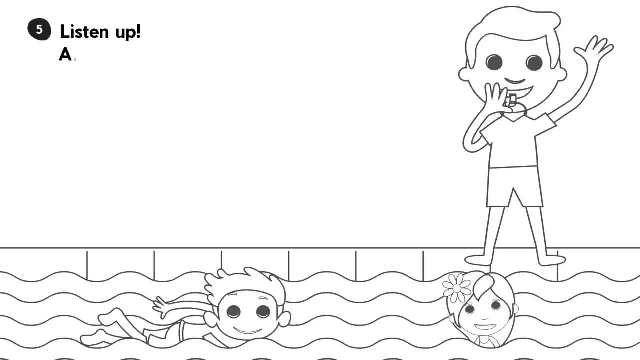 Rule number five is listen up At the pool. the lifeguards are in charge. So just like you have to listen to the babysitter when your parents aren't home, you have to listen to the lifeguard at the pool, And if you don't listen, they can make you get out of the pool. 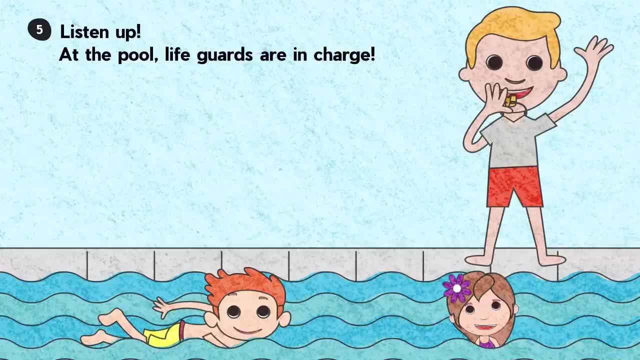 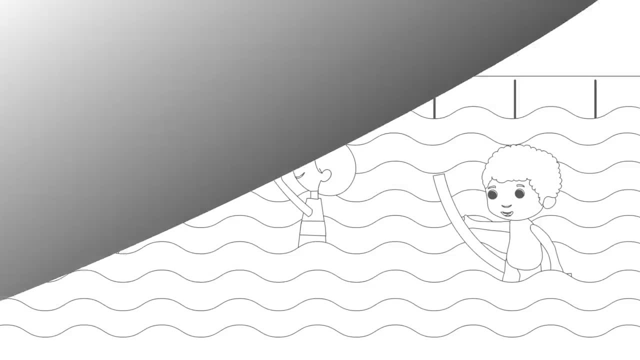 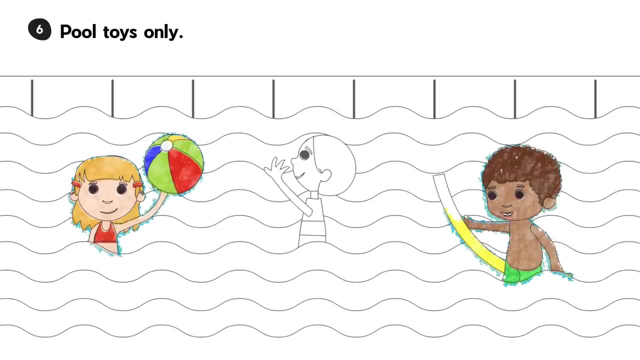 That's no fun. So when you're at the pool, who do you have to listen to? Yeah, The lifeguards. And rule number six is pool toys only In the pool. you have lots of great things you can play with, like noodles and beach balls. 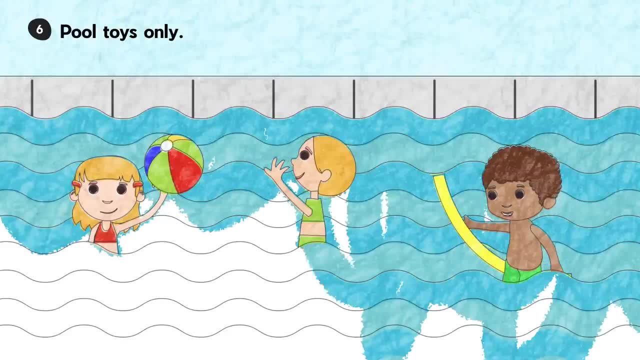 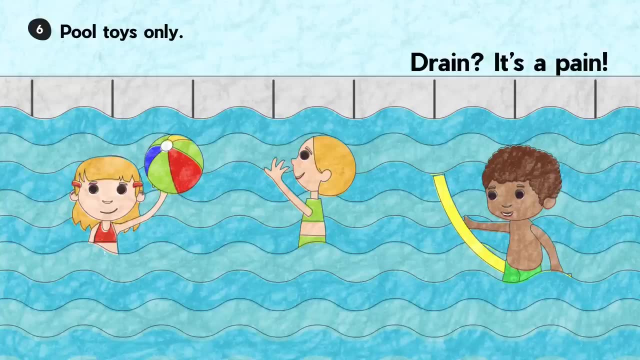 Don't toss other small toys on concrete. Throw all toys or coins in the pool because they can get stuck in the drain. And what is the drain? It's a pain, That's right. Is it okay to throw a tiny toy or coin into the pool? 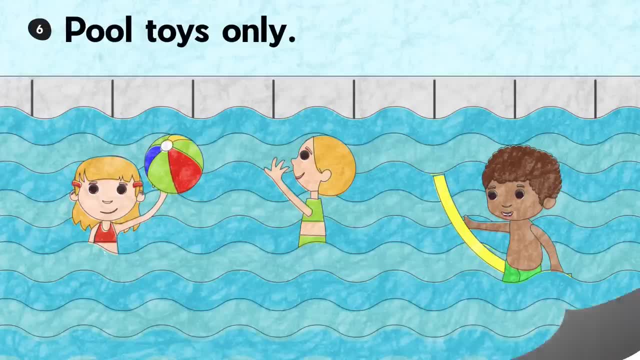 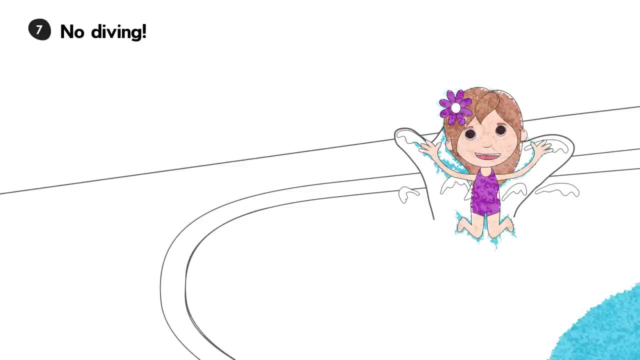 That's right. It's not Pool toys only. Rule number seven is no diving. You can really hurt yourself if you go into the shallow water head first and hit your head on the bottom of the pool. Feet first is the way to go. 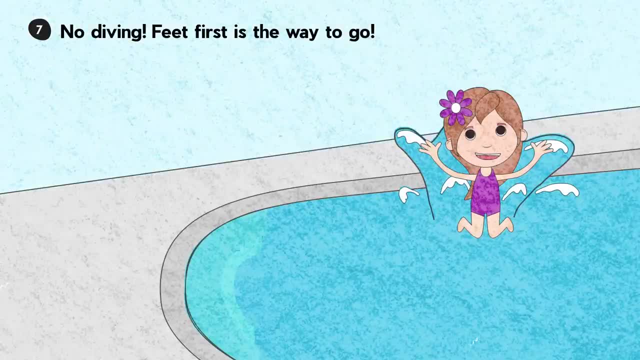 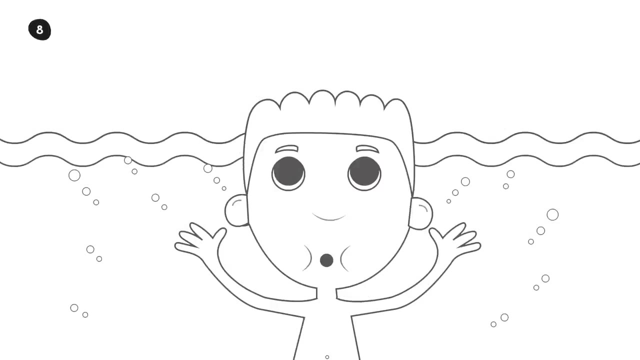 How should you go into the water? Exactly? Feet first is the way to go. Hey, is anyone here a fish? Anybody? No, I didn't think so. So rule number eight is to remember that fish can breed under the water. 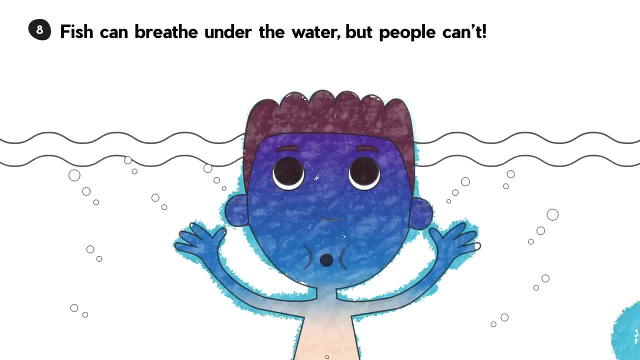 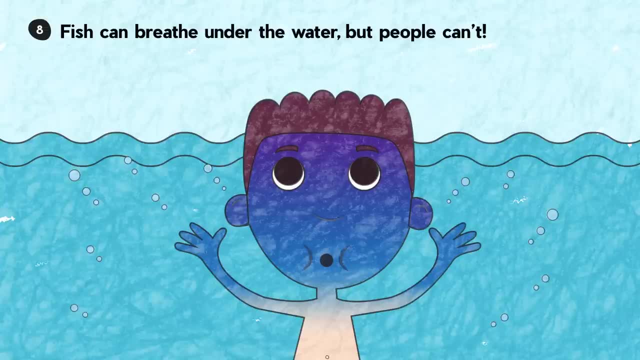 But people can't. So don't splash or dunk your friends a bunch of times in a row. Everybody needs a minute to catch their breath, even me. So what should we remember here? Are people fish? Nope, they're not. 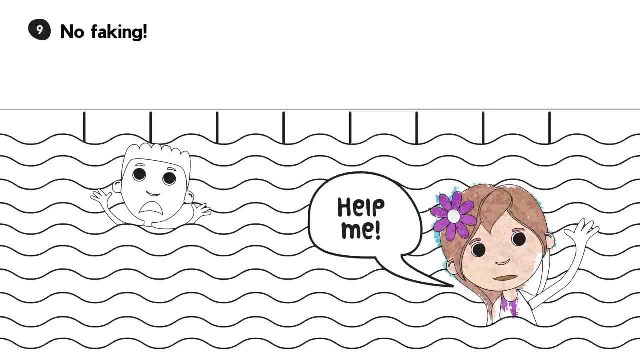 Rule number nine is no faking. Please don't ever pretend like you're in trouble in the water if you're not. It's scary for everyone if they think someone needs help, And it's one sure way to bring the fun to a stop.